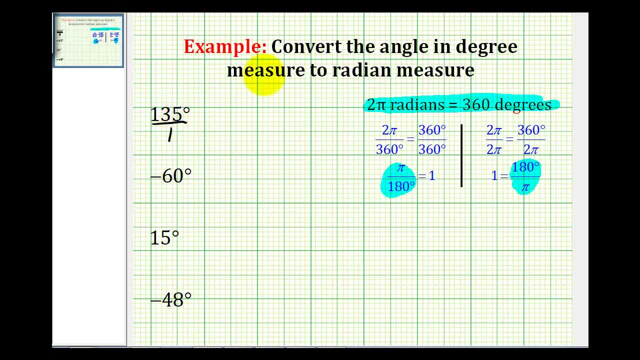 So we'll put it over 1. And we know if we want to convert degrees to radians we need to simplify out the degree measure, And we can do that if the degree measure is in the denominator. So we'll use this unit fraction to convert from degrees to radians. 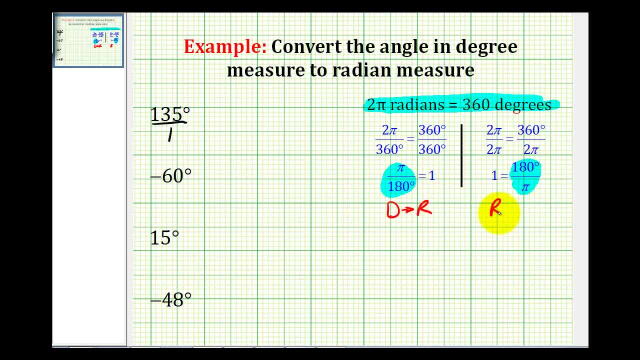 And we'll use this unit fraction in another video to convert from radians to degrees. So we're going to multiply all of these by pi divided by 180 degrees, And then we'll simplify and then we'll multiply. 135 and 180 have a common factor. 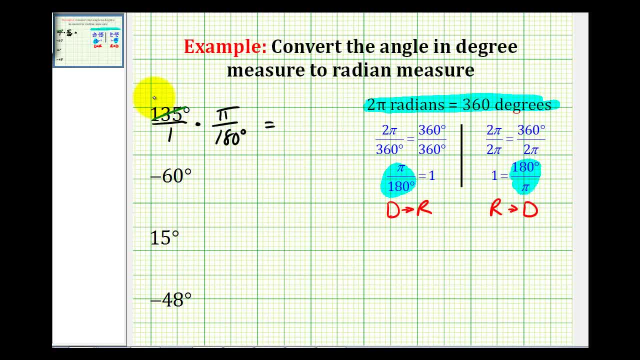 All right. So we have a common factor of 45. There are three 45s in 135, and there are four 45s in 180.. And the units of degrees also simplify out. So we're left with 3 pi divided by 4 radians. 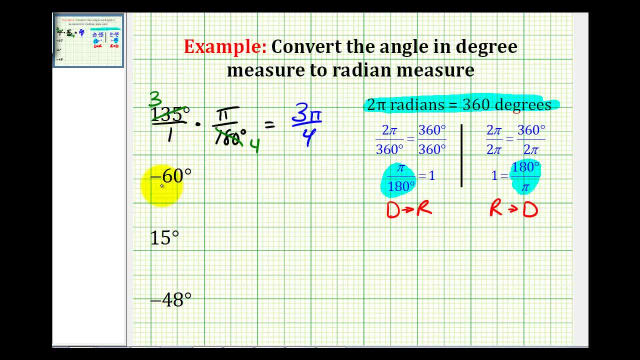 And we're going to do the rest of these the same way. But it is a fraction multiplied by pi, divided by 180 degrees. Here we have a common factor of 60.. All right, So there's 1, 60 in 60.. 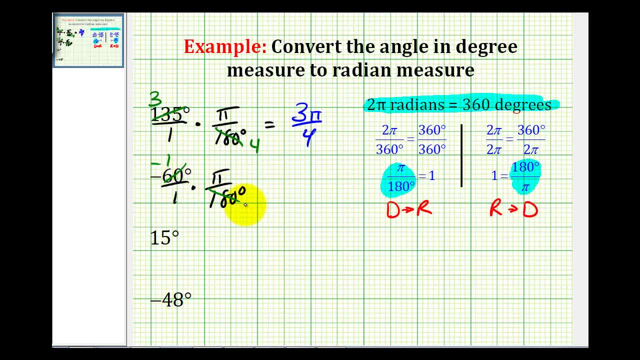 This simplifies to a negative 1.. There are three 60s in 180. And then again the degrees simplify out. So we're left with negative 1 pi divided by 3, or just negative pi divided by 3 radians. 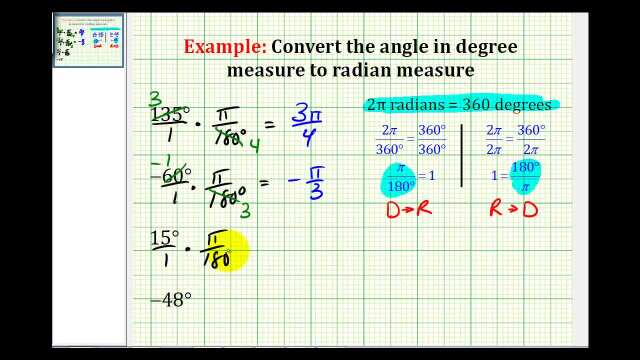 Put the 15 over 1,, multiply by pi over 180 degrees, Here we have a common factor of 15.. So this simplifies to 1.. And there are 12 15s in 180.. So we have 1 pi divided by 12, or just pi divided by 12 radians. 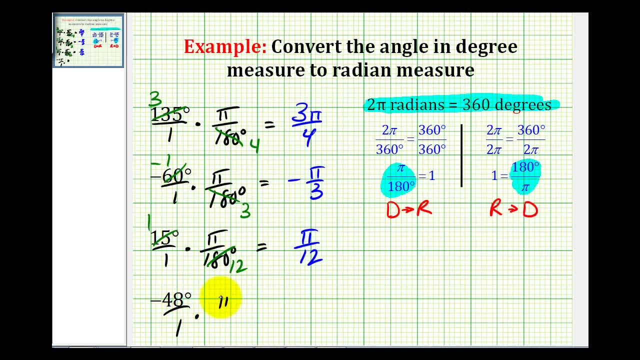 And we'll take a look at one more. 48 and 180 have a common factor of 12.. There are four 12s in 48, so this simplifies to negative 4.. And there are 15 12s in 180.. 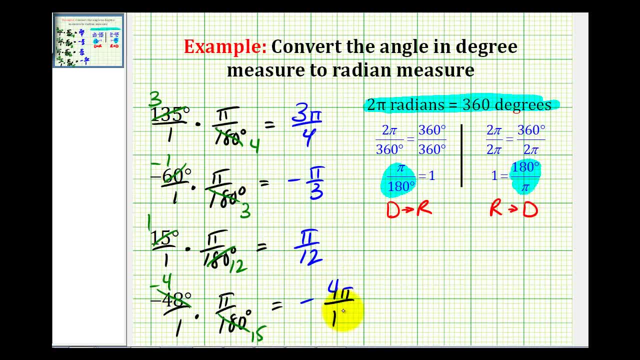 So here we have negative 4 pi divided by 15 radians. We've got three 남자 up on the right. Now, if we run the BM3, we'll get some baik. Notice how the bank looks like The broker has their this point. Now is the last, almost half banked. And what would be the profit кр? similar to medium 70.. A final Seung barrier. So here's the 양 arm, All right, And then together.